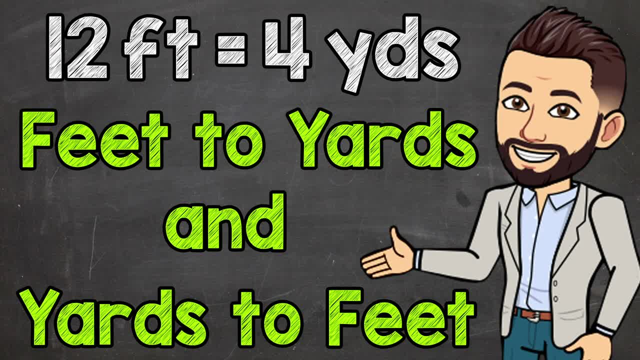 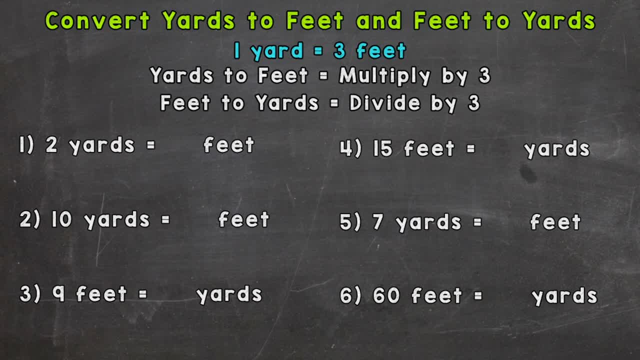 Welcome to Math with Mr J. In this video I'm going to cover how to convert yards to feet and feet to yards. So, as you can see on your screen, we have six conversions or problems that we are going to go through together. 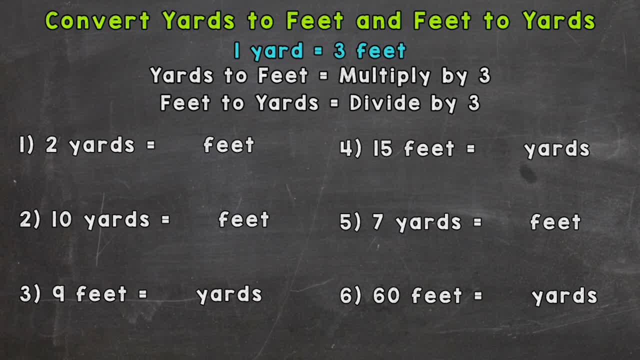 in order to help you get this down. Now, if you take a look at the top of your screen, I have some notes that you can reference as we go through these conversions. Now, your ultimate goal would be able to do feet to yards or yards to feet without those notes, but they are helpful to start. 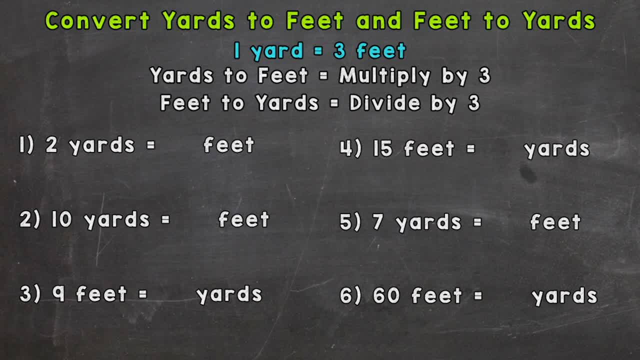 off. So let's jump right into number one here, where we have two yards equals how many feet? Well, if we take a look up top in the blue, we know that one yard equals three feet. So here we have two yards, So we're going yards to feet, So we need to multiply by three, So we need to do two. 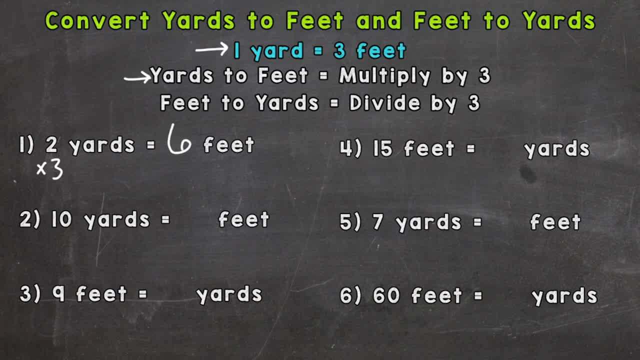 times three. So we need to do three times three, which gives us six feet. Now let's think about this one. Let's think yard sticks here One yard stick is three feet right. One yard equals three feet. Well, we have two yard sticks here, So three plus three. So that is two times the three. 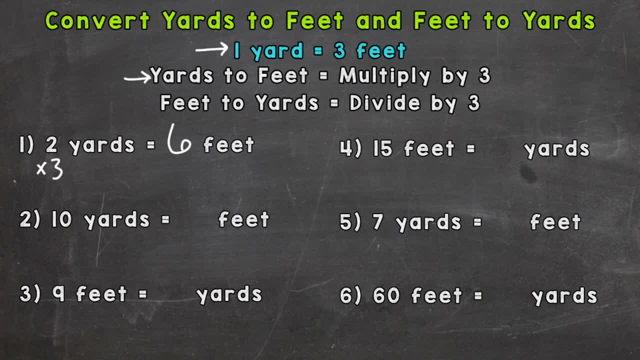 which we did there, gives us six feet. Let's take a look at number two. Ten yards equals how many feet? this situation: we would have 10 yardsticks, 3 plus 3 plus 3, 10 times, But it's easier to use. 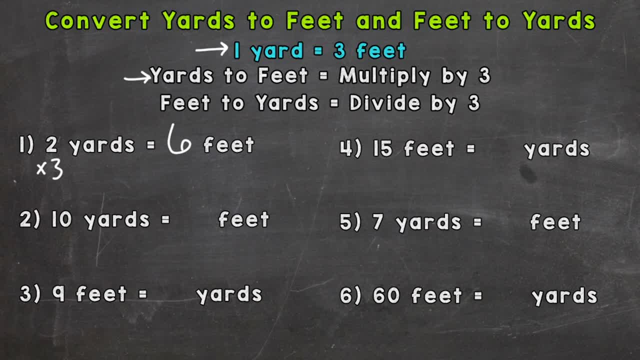 multiplication than add up 10, threes. So we can do again: yards to feet, we multiply by 3.. So 10 times 3 would give us 30 feet. Number three: we're going the opposite way. So we're going from feet. 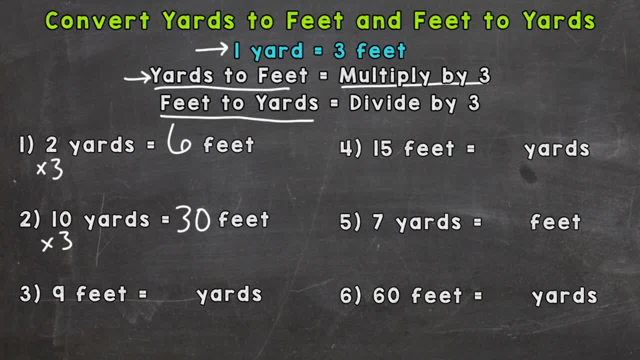 to yards, feet to yards. So we can think of it like this: We have 9 feet and we're splitting that 9 feet into groups of 3.. Each one of those groups of 3 is a yard, So we need to take that.